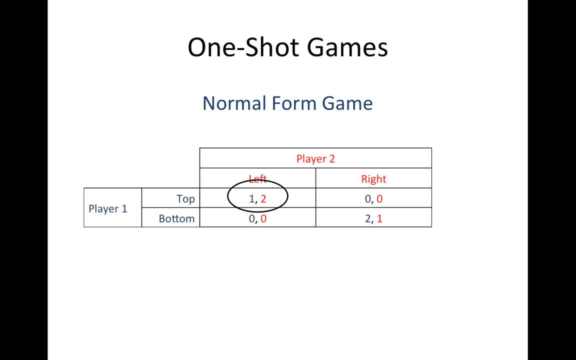 In this game, if player one plays top and player two plays left, then player one earns one and player two one. If player one plays top and player two plays right, then both players earn zero. If player one plays bottom and player two plays left, 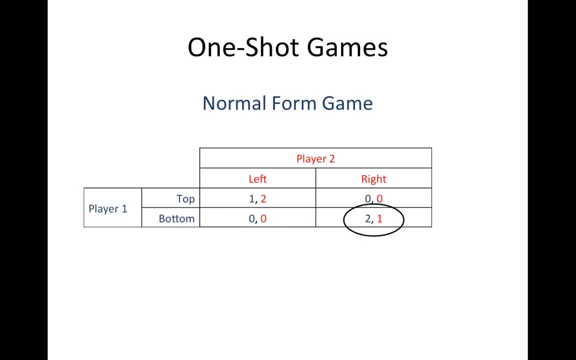 then again both players earn zero. And if player one plays bottom and player two plays right, then player one earns two and player two earns one. When considering how a player works and how a player will rank order outcomes from different actions, 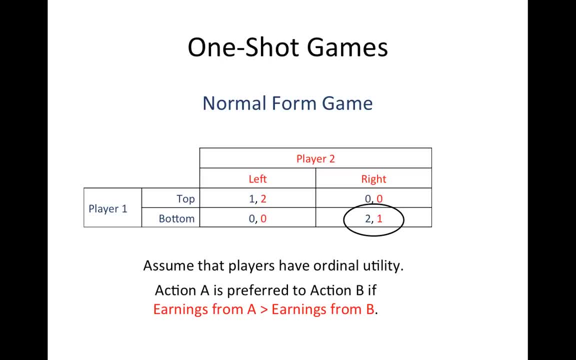 we assume that players have ordinal utility. This means that some action A will be preferred to some other action B if the earnings from action A are greater than the earnings from action B. Now that we know how to represent a game in normal form. 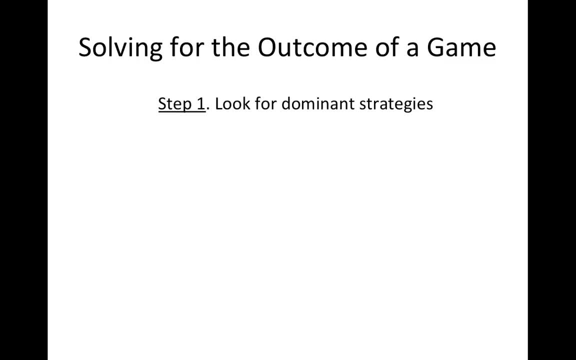 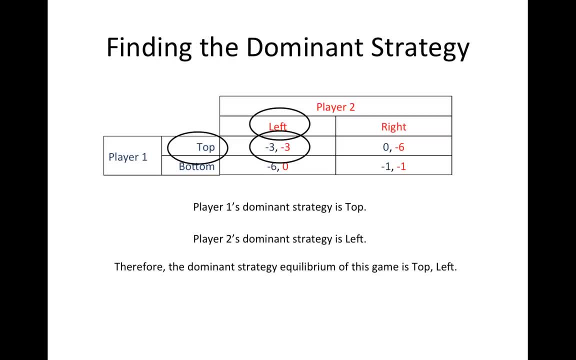 When this game have a dominant strategy. the dominant strategy equilibrium of this game is top left. This game is an example of a very special game known as the Prisoner's Dilemma. In this game, Player 1 and Player 2 are criminals who have been accused of a crime and placed 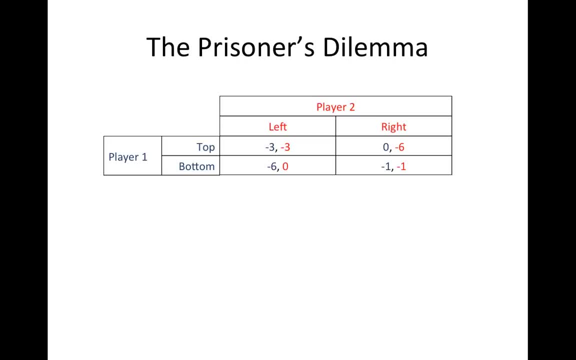 in different interrogation rooms. Each player's actions are either to confess the crime and implicate their associate, or deny that they committed the crime. If both players deny, then the prosecution only has enough evidence to convict them of a lesser crime and they each receive light sentences of one year. 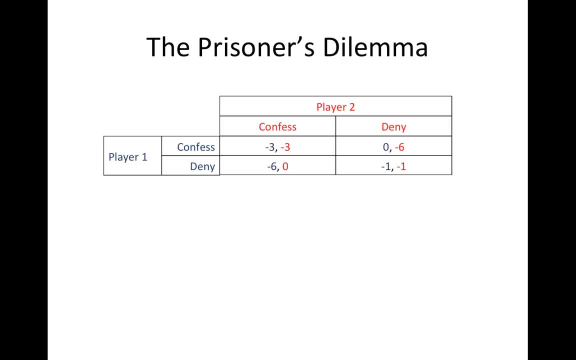 If one player confesses and one denies, then the player who confesses gets a plea deal and gets no time And the player who denies gets no time. The player who denies is convicted using the evidence provided by the confessor and gets six years. 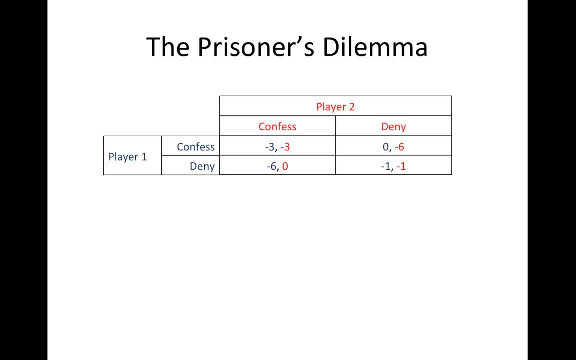 If both players confess, they receive an intermediate sentence of three years, Because both players have a dominant strategy to confess. this is the predicted outcome of the game. However, both players could be better off if they both deny, Because both players could be made better off by doing something different. the dominant 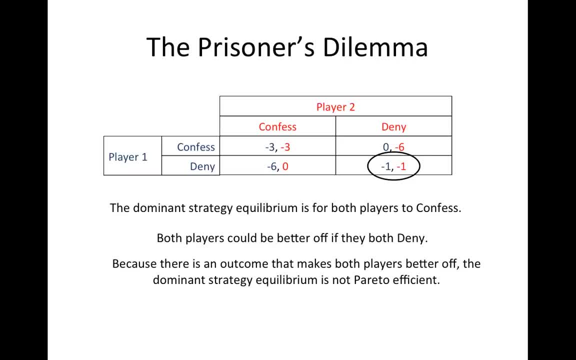 strategy equilibrium is not Pareto-efficient. The general class of games in which players playing their dominant strategy results in an inefficient outcome are known as Prisoner's Dilemma games. The Voluntary Contributions game in Public Goods Markets is an example of another game. 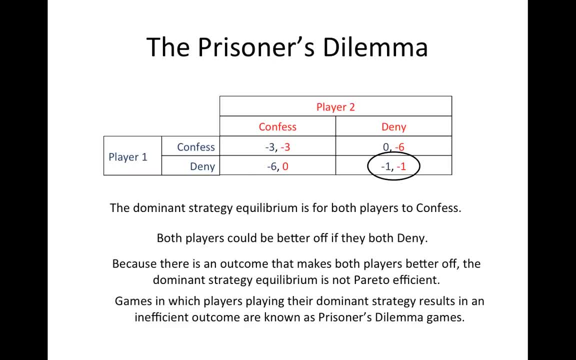 that has the same incentives and outcome as a Prisoner's Dilemma game. Sometimes, even though a player does not have a strategy to confess, the game is still a prisoner's dilemma game. The game is not a prisoner's dilemma game. 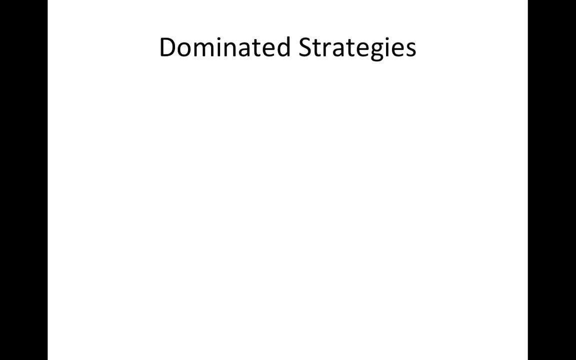 The disconsent or perfection of a prisoner's dilemma game is when a bad person is a prisoner's dilemma game. The game cannot be a prisoner's dilemma game if you have a penalty or cerebrum. clever standard ala. There are still only two players, but each player has three possible actions. 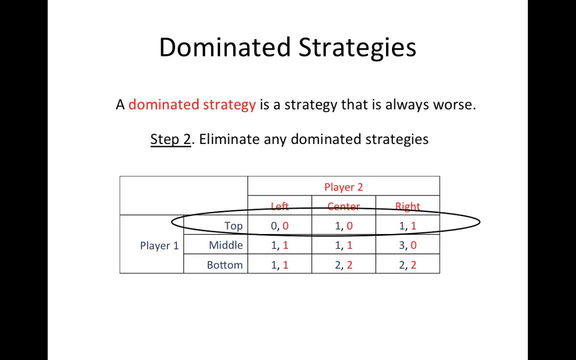 Let's start by considering Player 1.. For Player 1, playing top always gives earnings that are the same as or worse than both middle and bottom. Thus, for Player 1, we say that the strategy top is a weakly dominated strategy. 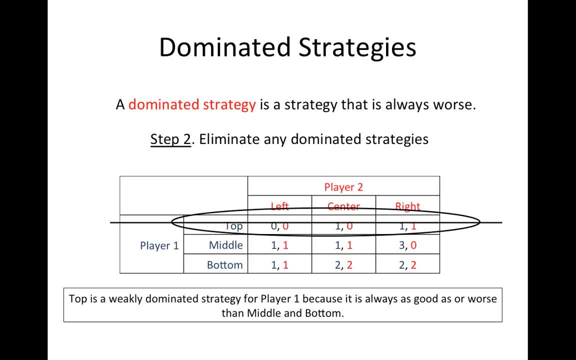 and we can eliminate it as one of the strategies that Player 1 is likely to play. Now that we have eliminated top, we should consider the game from Player 2's perspective, If Player 2 knows that Player 1 will never play top. 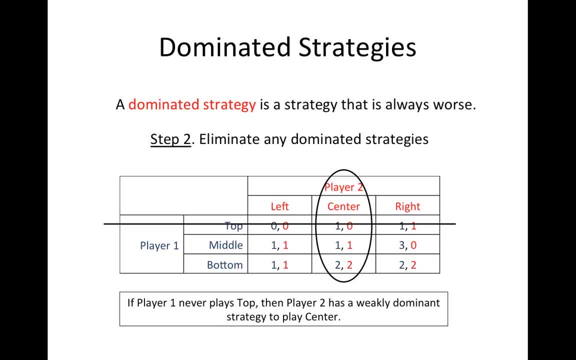 then for Player 2, center is always at least as good or better than either left or right. When this is the case, we say that Player 1 is likely to play top and Player 2 has a weakly dominant strategy to play center. 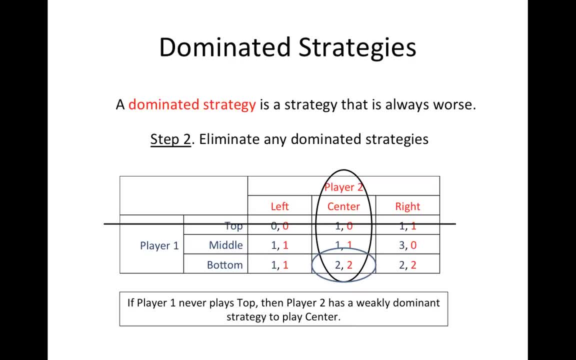 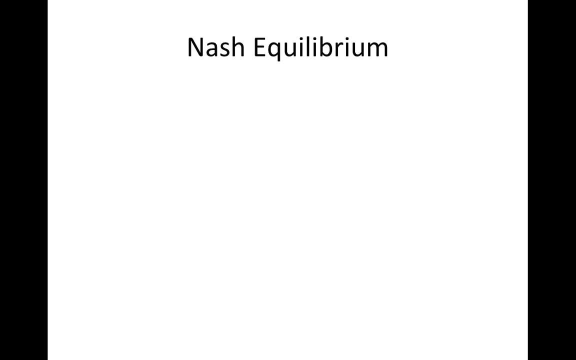 Given this, Player 1 should play bottom. Therefore, by eliminating dominated strategies, we have found the equilibrium outcome of this game. If we cannot find an outcome of the game by identifying dominant and dominated strategies, then Step 3 of the analysis is to look for a Nash equilibrium. 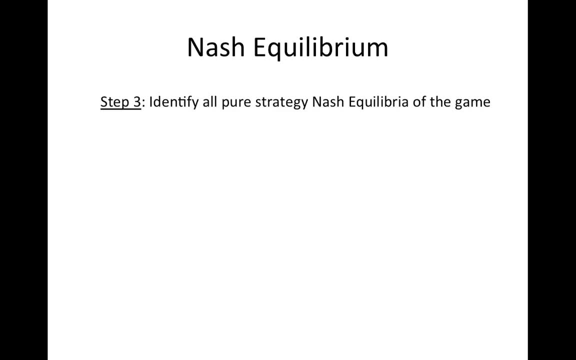 We start by identifying the equilibrium outcome of the game. We start by identifying all pure strategy Nash equilibria of the game. If a player is playing a pure strategy, then they are choosing one strategy and sticking to it. Contrast this with a mixed strategy. 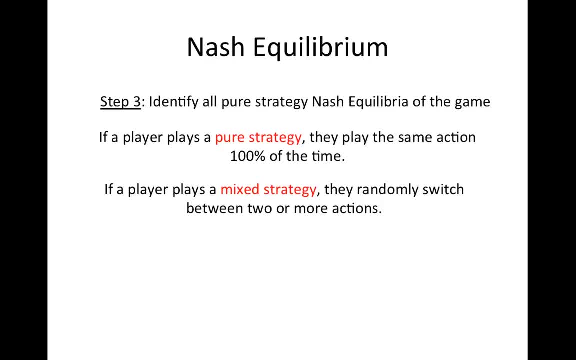 in which a player randomly chooses between two or more actions, An outcome is a Nash equilibrium. if Player A's action is an optimal response to Player B's action and Player B's action is an optimal response to Player A's action, Player B's action is simultaneously an optimal response to Player A's action. 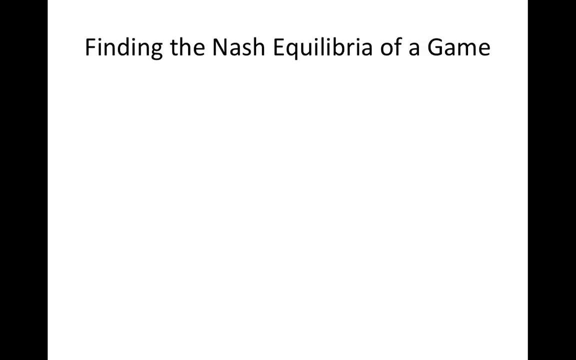 Let's consider a couple of examples to see how to find the Nash equilibrium of a game. To find the pure strategy Nash equilibrium of a game, start by asking yourself this question for each outcome. At this outcome, given what the other player is doing, 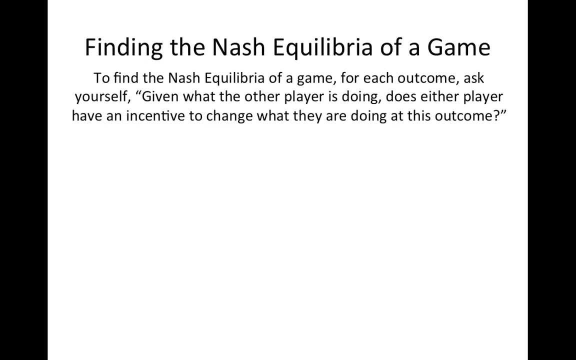 does, either player has an incentive to change what they are doing. If the answer is yes for either player, then that outcome is not a Nash Equilibrium. If the answer for both players is no, then the outcome is a Nash Equilibrium. Let's consider the example from the start of this presentation. 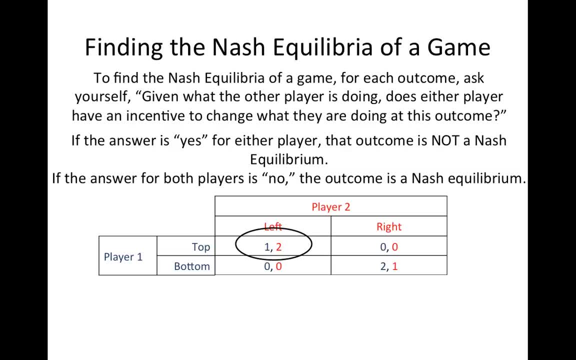 Let's start with the outcome: top left. Does either player have an incentive to change what they are doing at this point, given what the other player is doing? Given that player 1 is playing top, player 2 does not have an incentive to change from left to right, since they will earn 0 instead of 2 if they change. 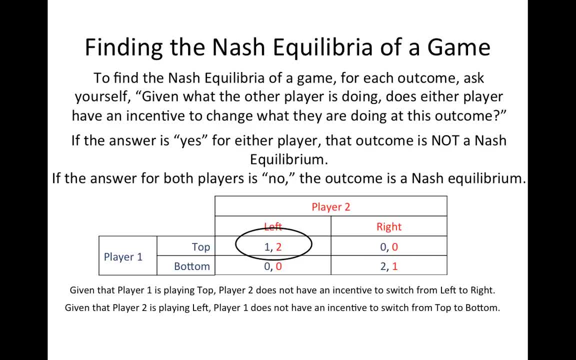 Similarly, given that player 2 is playing left, player 1 does not have an incentive to change from top to bottom. Since neither player has an incentive to change what they are doing, the outcome- top- left- is a Nash Equilibrium of this game. 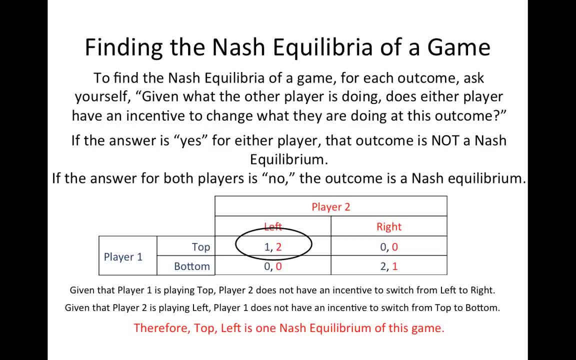 However, it is not necessarily the only Nash Equilibrium of the game, so we should consider the other outcomes as well. We can easily rule out top right, since both players have an incentive to change what they are doing at that point. We can rule out bottom left using a similar logic. 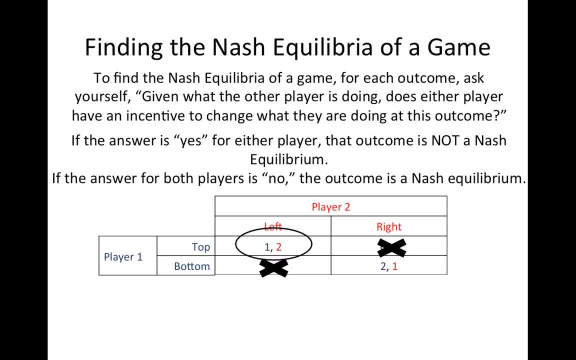 We have one more outcome to check, which is bottom right. If player 1 is playing bottom, player 2 does not have an incentive to change from bottom to right, since they will earn 0 instead of 2 if they change. If player 2 is playing bottom, 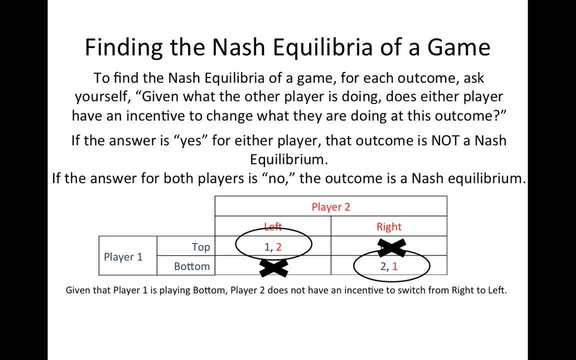 player 2 does not have an incentive to switch from right to left. Similarly, if player 2 is playing right, player 1 does not have an incentive to switch from bottom to top. Therefore, this outcome is also a Nash Equilibrium. 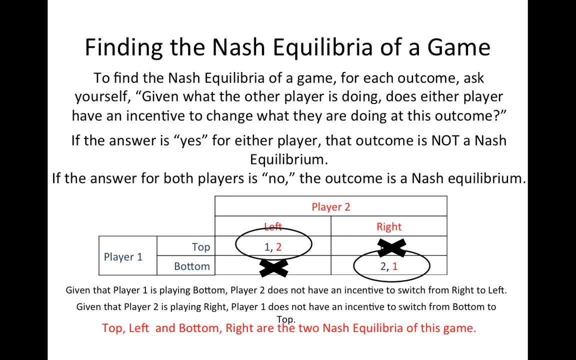 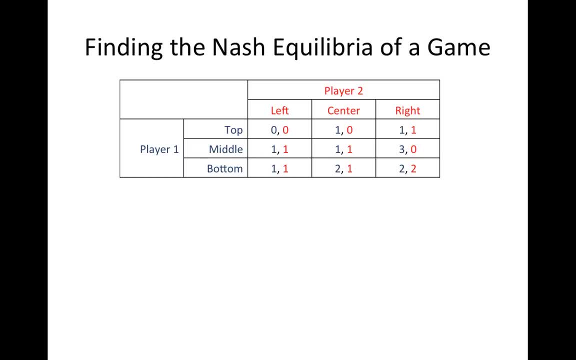 We have found that this game has two Nash Equilibria: top left and bottom right. Let's do one more example that's a bit more complicated. This game is similar to the two-player three-action game that we examined earlier, except that some of the earnings have changed slightly. 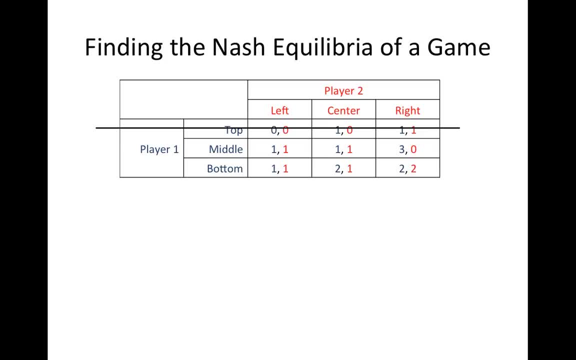 We know from earlier that top is a dominated strategy for player 1, so, to make our lives easier, we'll eliminate all outcomes involving player 1 playing top from consideration, since we know that all these outcomes, player 1 has an incentive to change what they are doing. 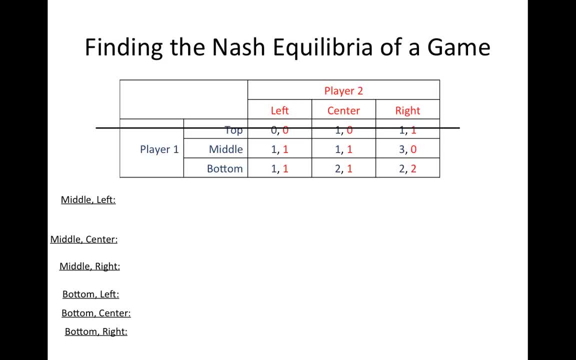 We have six outcomes to consider. Let's start with Nash Equilibrium. Let's start with middle left. If player 1 is playing middle, player 2 does not have an incentive to change to either center or right. Similarly, if player 2 is playing left, 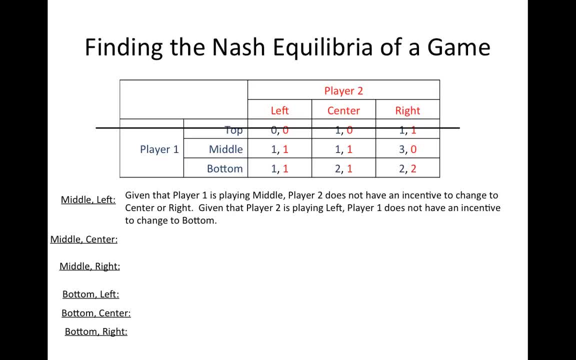 player 1 does not have an incentive to switch to bottom. Therefore, middle left is one Nash Equilibrium of this game. If we consider middle center, at this outcome, given that player 2 is playing center, player 1 has an incentive to switch to bottom. 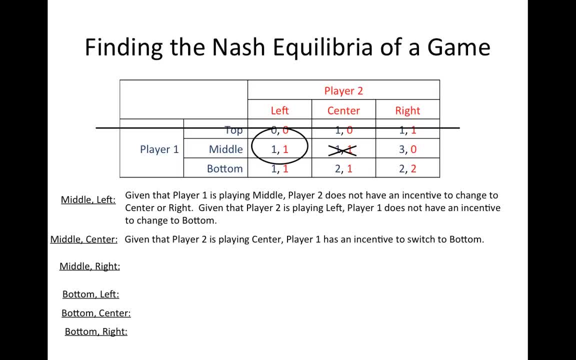 so this outcome is not a Nash Equilibrium. At middle right, given that player 1 is playing middle, player 2 has an incentive to switch to either left or center, so this outcome is not a Nash Equilibrium either. At bottom left, given that player 1 is playing bottom. 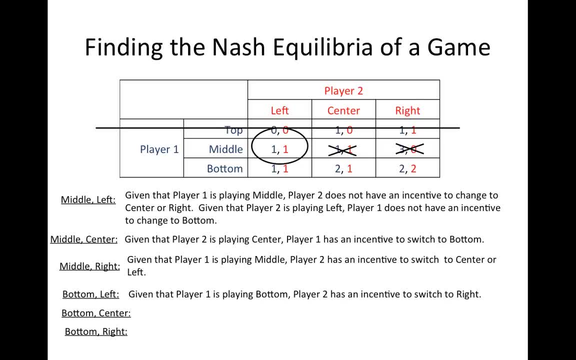 player 2 has an incentive to switch to right, so this outcome is not a Nash Equilibrium. At bottom center, player 2 also has an incentive to switch to right, so this outcome is not a Nash Equilibrium. Finally, at bottom right, given that player 2 is playing right. 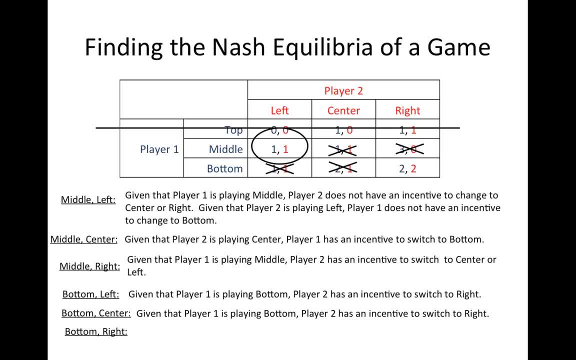 player 1 has an incentive to switch to middle, so this outcome is not a Nash Equilibrium. Therefore, we have found that this game has a unique pure strategy Nash Equilibrium of middle left. What if we don't find any pure strategy equilibria for a game? 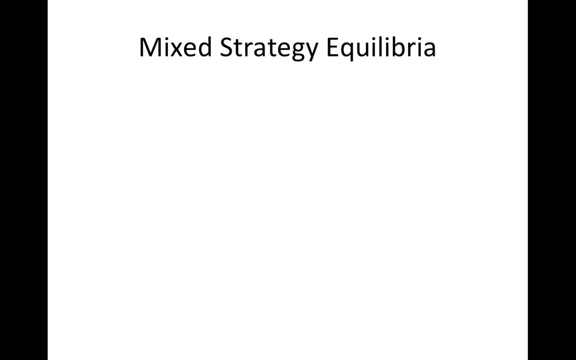 or we find multiple pure strategy equilibria. In this case, we can also look for mixed strategy equilibria. In a mixed strategy equilibrium, players randomly choose between two or more strategies. The key to finding a mixed strategy equilibrium is to note that in such an equilibrium, 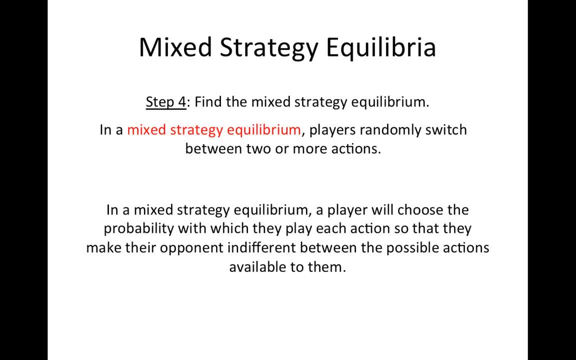 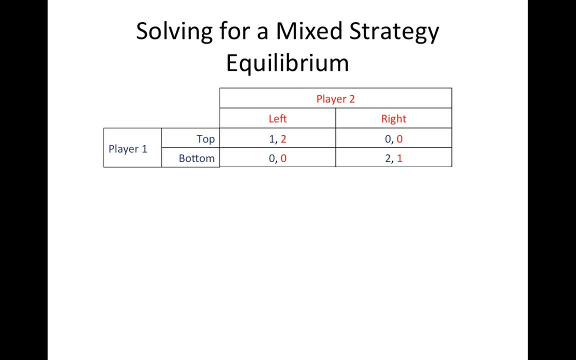 each player will choose their strategies in such a way as to make their opponent indifferent between their possible choices. Let's consider an example. In this game, we found that there were two pure strategy Nash Equilibria: top left and bottom right. In a game such as this, 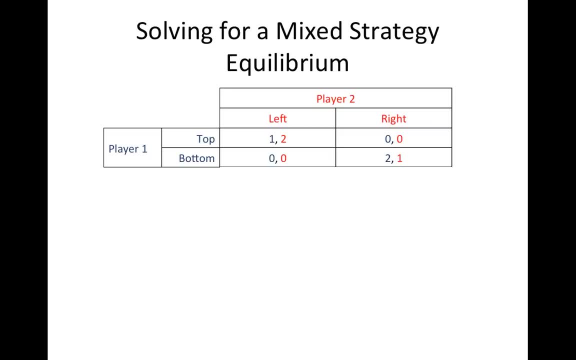 there will also be a mixed strategy equilibrium. Let's let P be the probability with which player 1 chooses top, which means that they will choose bottom with probability 1-P. Player 1 wants to choose P to make player 2 indifferent between playing left and right. 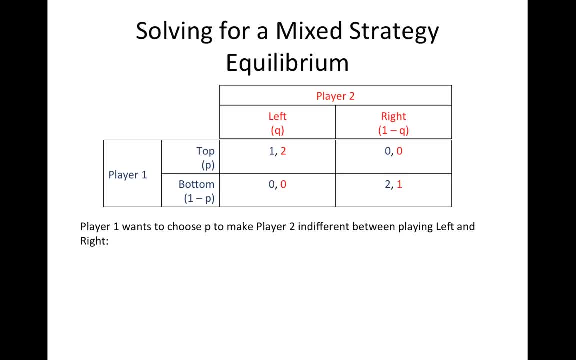 If player 1 plays top with probability P and bottom with probability 1-P, player 2's expected earnings from playing left are 2P. Player 2's expected earnings from playing right are 1-P. To make player 2 indifferent between these two choices, 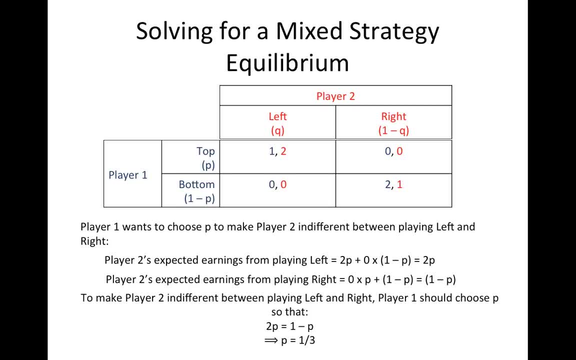 player 1 should choose P, so that player 2's expected earnings from the two choices are the same, which means that 2P equals 1-P. If we solve this equation for P, we find that player 1 will play top, with probability 1-3. 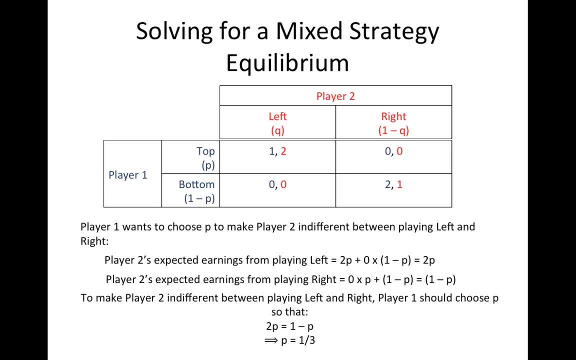 and bottom, with probability 2-3.. We can conduct a similar analysis to find player 2's optimal strategies. Player 2's probability of playing left is Q and their probability of playing right is 1-Q. Player 2 should choose Q. 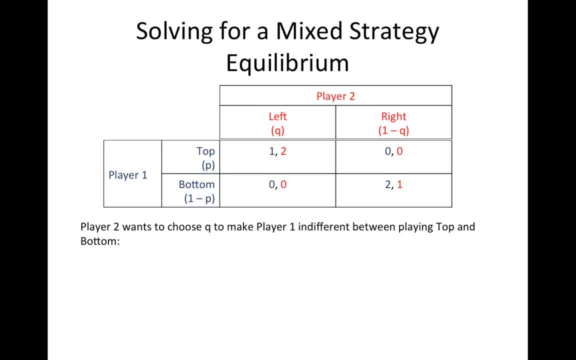 in order to make player 1 indifferent between playing top and playing bottom, Player 1's expected earnings from playing top are equal to Q. Player 1's expected earnings from playing bottom are 2 times the quantity 1-Q. In order to make player 1 indifferent. 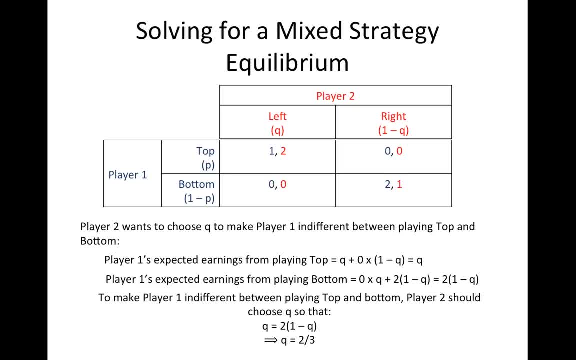 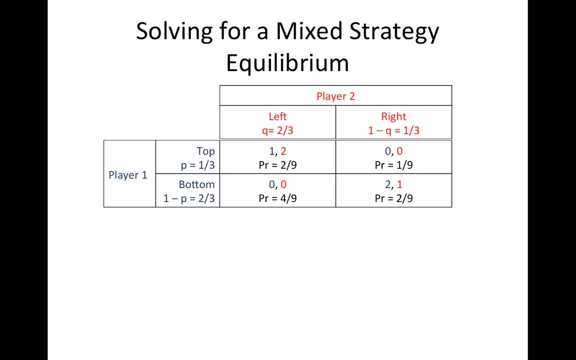 between playing top and playing bottom. player 2 should play left with probability 2-3, and right with probability 1-3.. When we combine each player's mixed strategy, we have found the mixed strategy equilibrium of the game. So far in all of the games that we have studied. 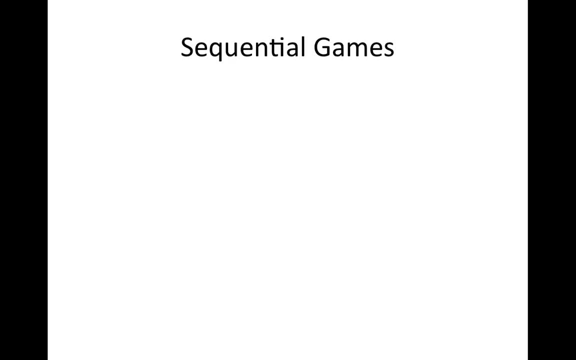 players make their choices simultaneously. In many strategic situations, players make their choices sequentially. To represent a sequential game, economists often use the extensive form of a game. An extensive form representation of a game is simply a tree. We put the player who goes first. 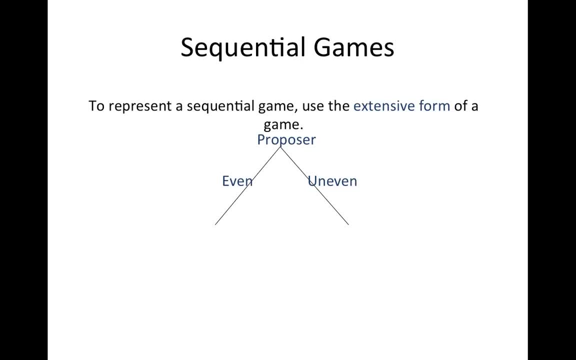 at the first node of the tree and create a branch for each of player 1's possible actions. The player who goes second goes at the end of player 1's branches, with his possible actions as branches as well. We put the earnings for each player. 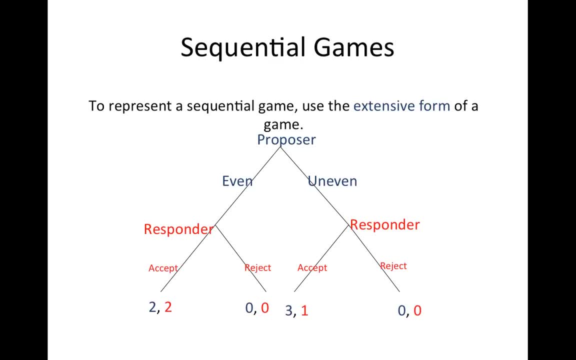 at the ends of the branches, following the convention that we list the first mover's earnings first. Color has been added to this diagram to help you link players' actions and earnings To solve sequential games we use a process called backward induction. With backward induction, 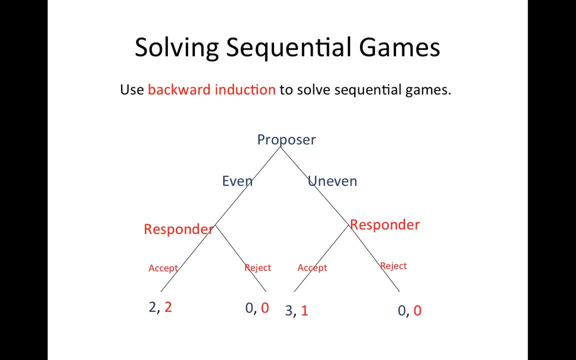 we start by determining the optimal strategy for the player who goes last and then, given this, determine the optimal strategy for the player who moves first. The game represented in this diagram is a version of a game called the proposer-responder game. 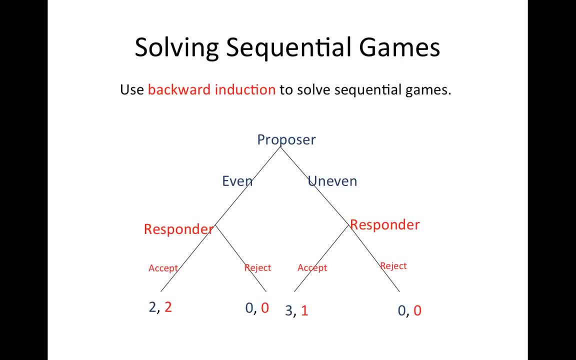 This game can be generalized to apply to all sorts of games or all sorts of negotiation situations. In this game, the proposer has $4, which he can decide to divide either evenly or unevenly. Once the proposer announces the division, the responder can either accept. 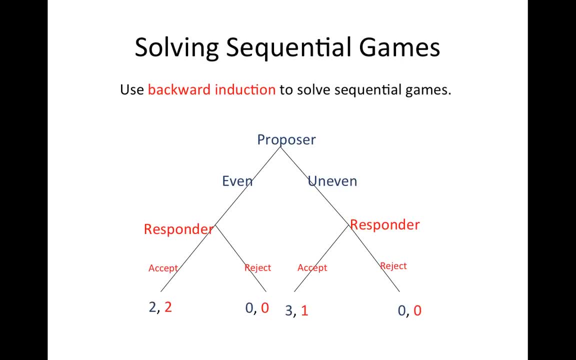 or reject the proposer's offer. If the responder accepts, the money is divided according to the proposer's chosen decision. If the responder rejects the proposal, both players get zero. We can see that in this game, the responder's optimal choice.